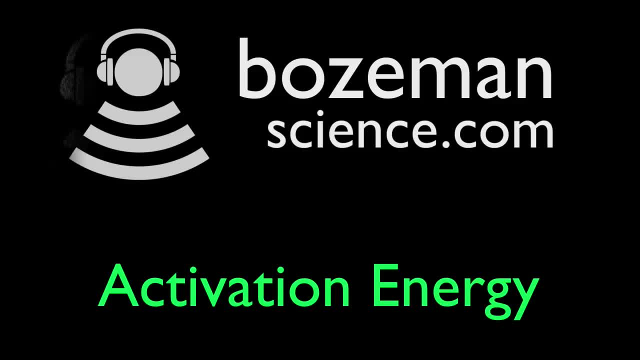 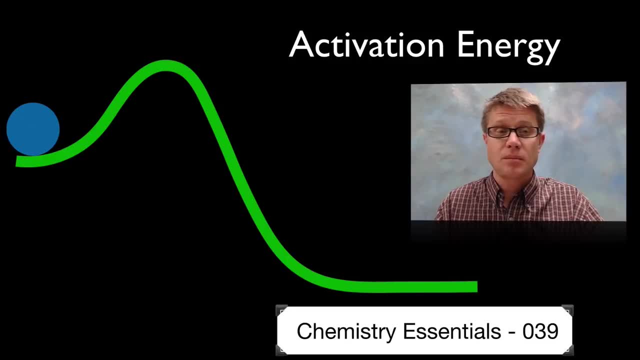 Hi, It's Mr Andersen, and this is chemistry essentials, video 39. It's activation energy. Imagine if I try to roll a ball up a hill. If I get enough energy into that system, the ball is going to roll down the other side. In other words, there was a certain amount. 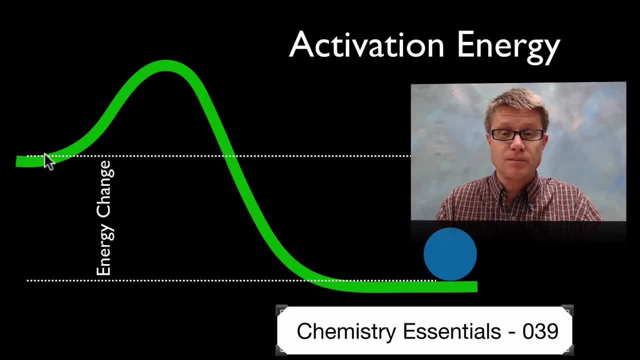 of energy that that ball had at the beginning. We'll call that potential energy. And then we've lost some of that potential energy. But the ball just didn't go there on its own. I had to put a certain amount of energy into it And in chemistry we call that activation. 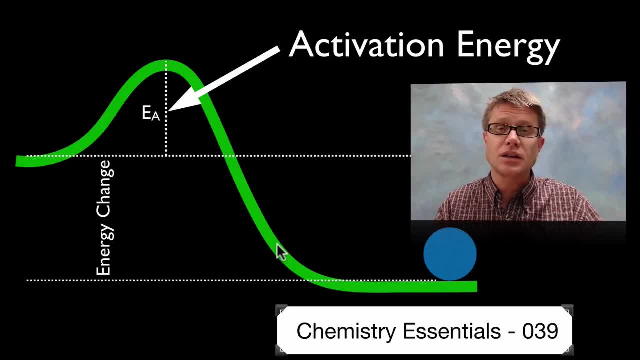 energy Now it's not only balls rolling up a hill and down the other side, It's chemical reactions. You can think of this as the reactants on this side And this as products on the other side, And so we're only netting this amount of energy between here and here. But 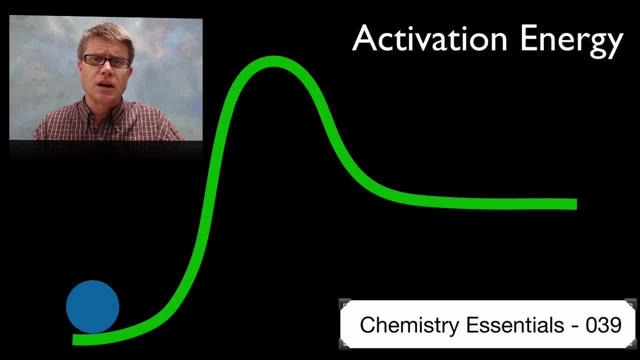 there's energy that you have to put into the system. Let's say we have an endergonic reaction like this One that requires energy. Well, I'm going to put more energy in. I'm going to get some of that back. If we were to look at the energy change, then everything above that is going to be the activation. 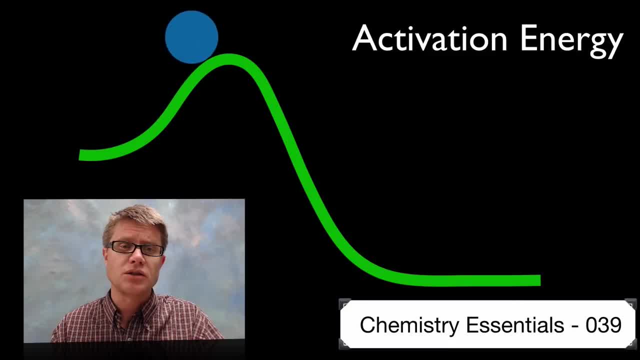 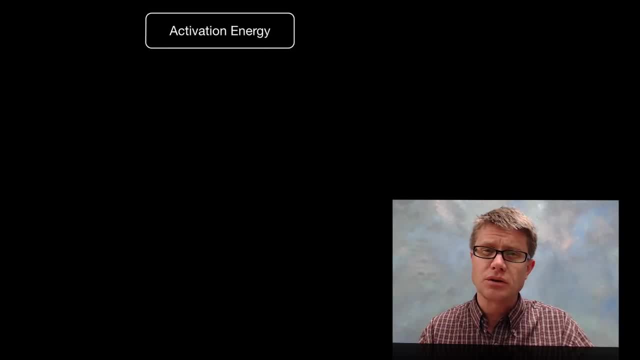 energy. What if I don't have enough activation energy? Well, I can put some energy in, But if I don't have enough, then it's going to go back to where it was before, And so activation energy is how much energy you have to put into a system to have a chemical reaction. 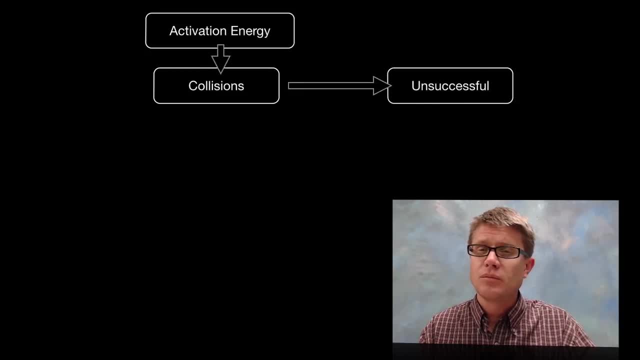 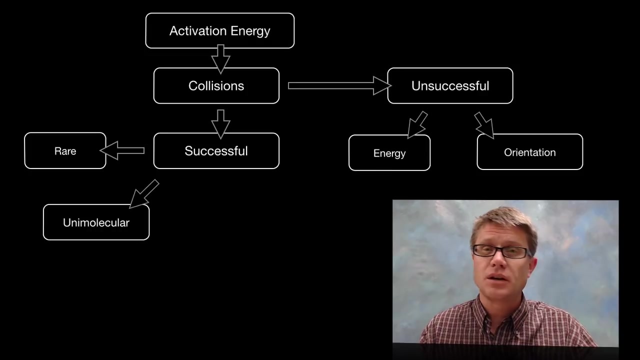 occur And it's based on collisions between molecules. Most of those are unsuccessful collisions And that's because they maybe don't have enough energy or they don't have proper orientation. But if they are successful- which again is incredibly rare- then we can have chemical reactions fire off In a unimolecular reaction. 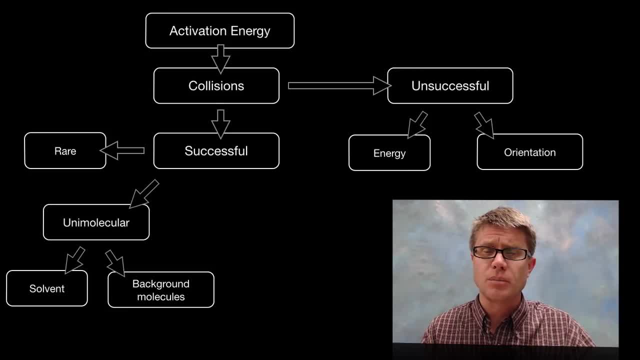 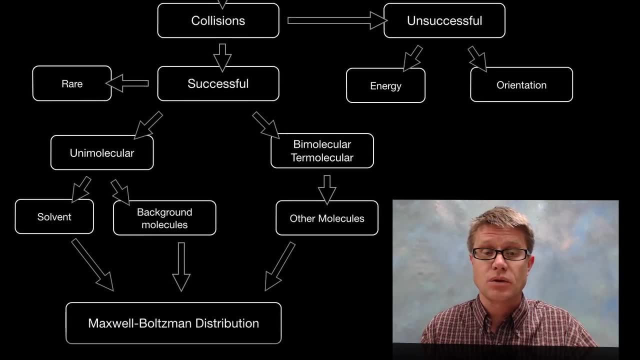 that's mostly going to be interactions between the molecule and the solvent or background molecules. But if it's a bimolecular or termolecular reaction, it's going to be with other molecules or reactions with other molecules. In either case, it's going to be based on the Maxwell. 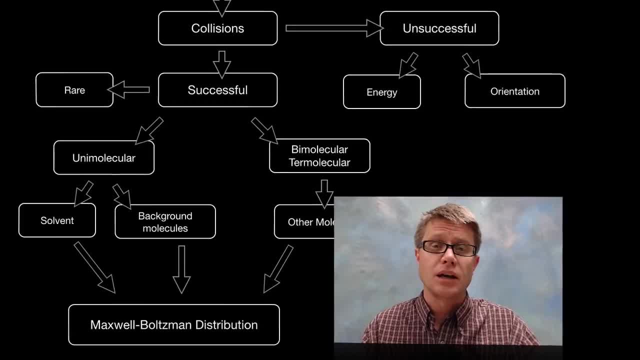 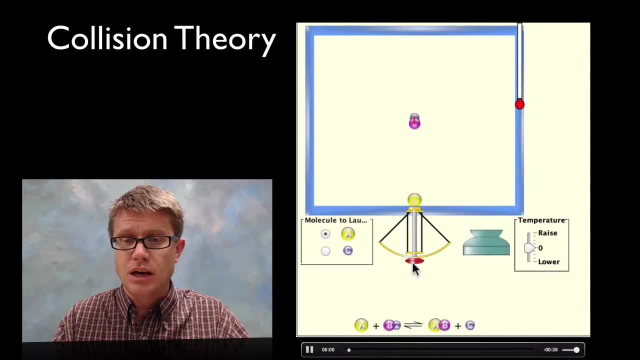 Boltzmann distribution, How often this is going to occur. And again, that's where we can determine activation energy. And so let's say we have two molecules. We'll call this A and B. And if I were to launch A at B, what we'll find is that if I don't give it enough, 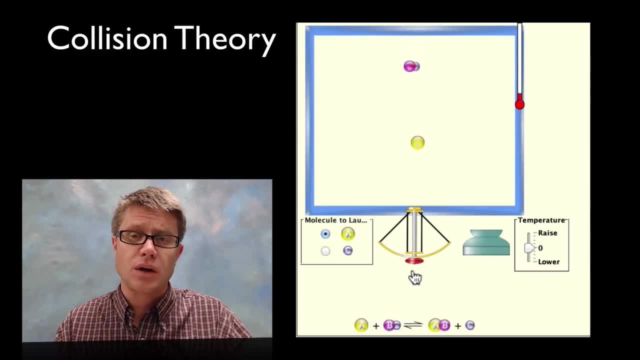 energy, then there's not going to be a chemical reaction in this one simple collision. In other words, you require a certain amount of energy for that reaction to occur. So it's kind of based on temperature. If I increase temperature I can have more reactions Also. 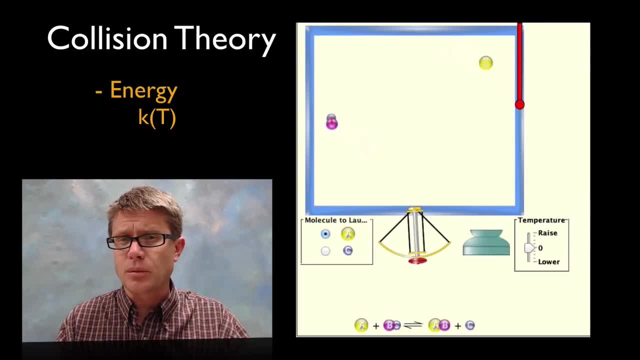 if I fire it off center like that, then they're not lined up properly and there's not going to be a reaction as well. And so with each of these collisions between all of the molecules, you have to make sure that you have proper energy and you also have proper orientation. But if you do, then we can fire off that reaction. 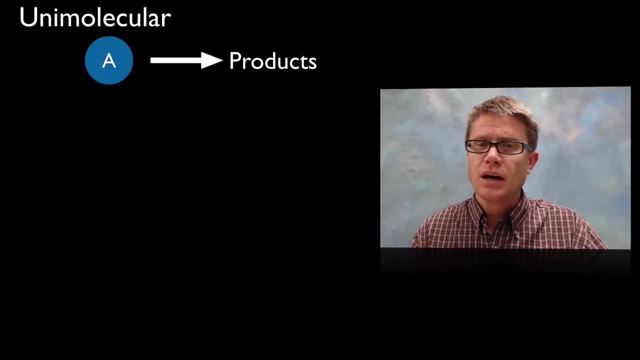 In other words, we've exceeded that activation energy, And so this could be in a unimolecular, when we have just one molecule turning into products. It could be bimolecular, where they're running into each other, Or it could even be termolecular. We have three things coming. 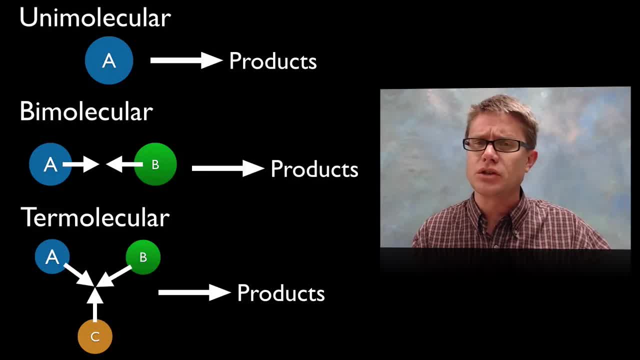 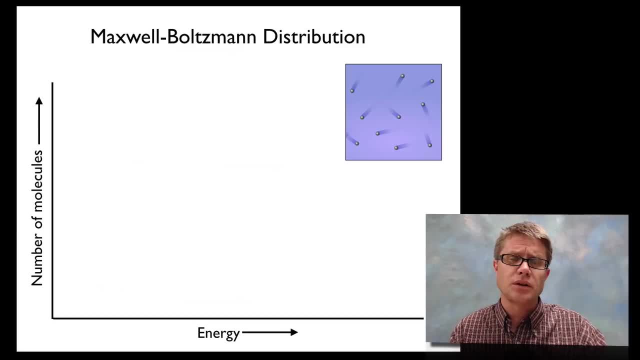 together at once, And so all of these are based on the number of collisions that we could possibly have, And so the Maxwell Boltzmann distribution distribution explains how much energy we have to put into a system for that chemical reaction to actually occur, And so the curve looks like this, And so let me explain it to you. 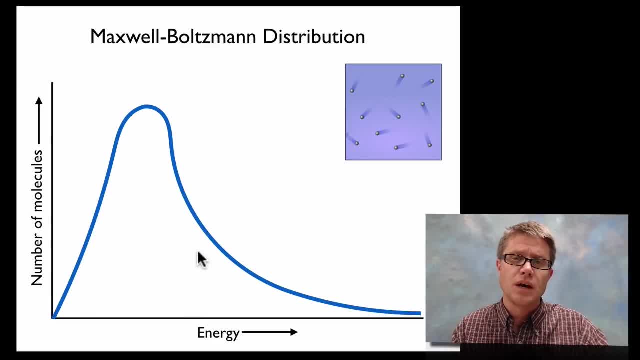 If you think of this curve representing all the molecules that have a potential to interact, well, we'd say the mode is going to be right here. This is the number that have this amount of energy and this is the number of particles that we have If we look on the left side. 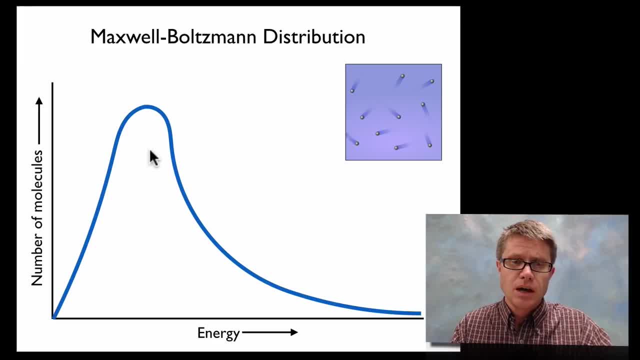 right down here there are going to be no particles who have no energy. And then, as we move to the right side, the mean is going to be a little bit to the right of that, Because there's going to be a lot of particles way out here that have a huge amount of energy. Now there's 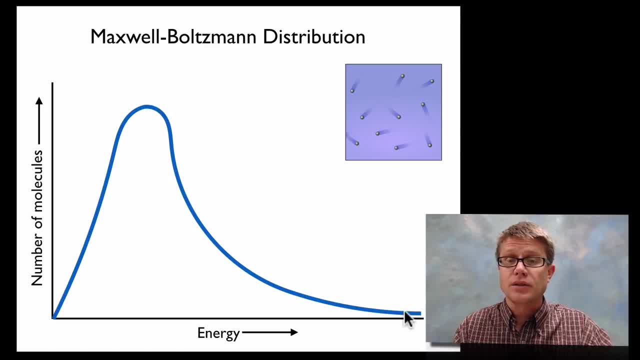 not many of those particles out there, But there's a lot of particles out there that have quite a bit of energy, And so if we look at that area under the curve, that represents all the molecules that we have or have the potential to have interactions with, And so 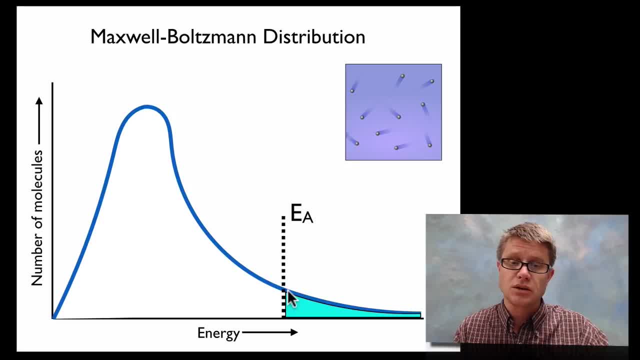 we're going to set E sub A right here. That's going to be that activation energy, And so all of these out here have the proper amount of energy to actually have a potential to have a chemical reaction occur. And so what happens if we increase the temperature? 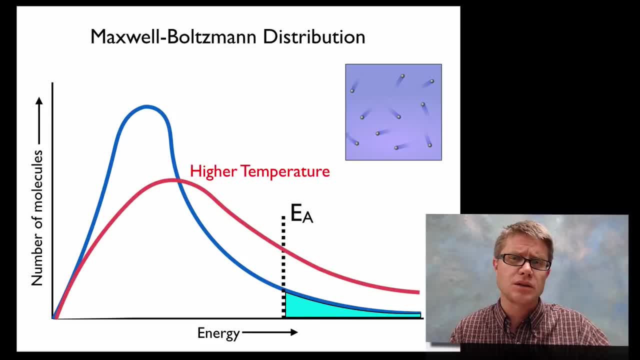 Well, if we increase the temperature, we just get a different curve. It's going to be the same number of particles, But it's shifting everything to the right. Notice what happened to the activation energy. The activation energy still is the same. It still requires a certain